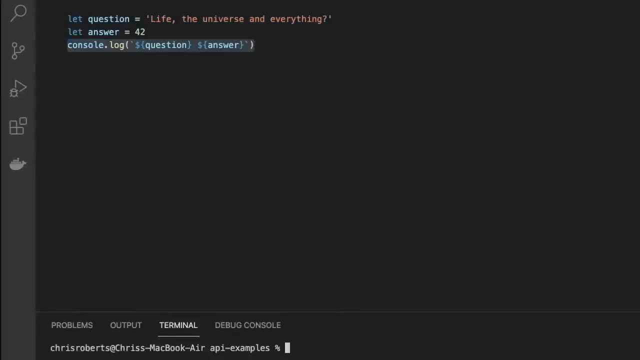 JavaScript, such as strings and numbers. our code executes sequentially. We can assign a string, a number and then combine the two values together straight away. Everything is nice and simple. However, when writing real-world code, we often make calls through databases, open files. 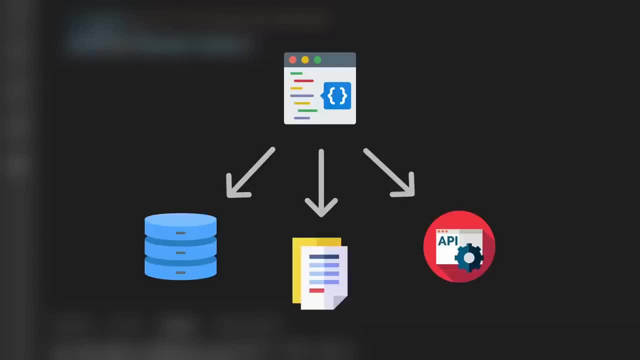 and speak to remote APIs over the internet. Longer-running tasks like this will usually not return the results straight away. They will rather return a promise. A promise is a special type of object in JavaScript that represents the eventual completion or failure of an asynchronous operation and its resulting value. If this sounds a little bit hard to understand, maybe we can. 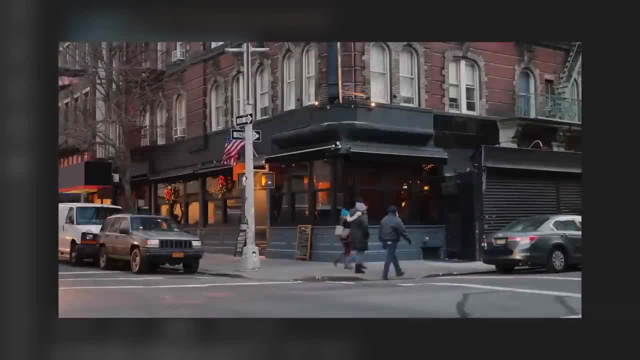 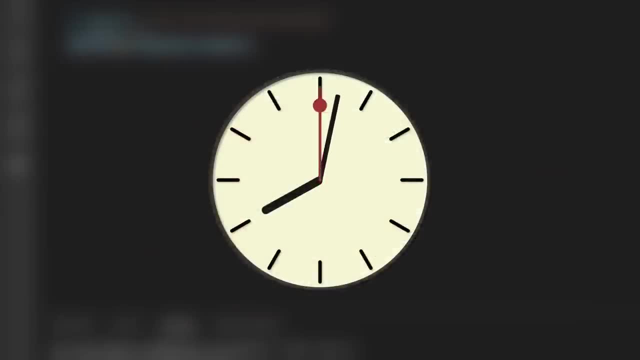 imagine it as a real-world scenario. Imagine you are at a restaurant having dinner and you ask the waiter to bring you another cup of coffee. The waiter promises to come back with your coffee. However, you can't drink it at that point. You have to wait until he returns with your coffee. 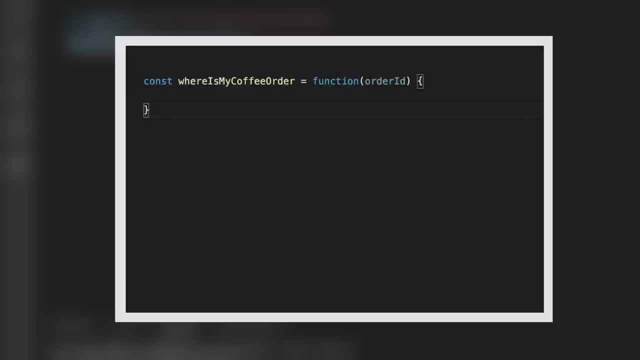 and the promise is fulfilled. and this is the same sort of concept in JavaScript. If, for example, you request some information from a remote API, then you will be immediately given a promise that task will eventually either complete or fail. It's not until some time later. 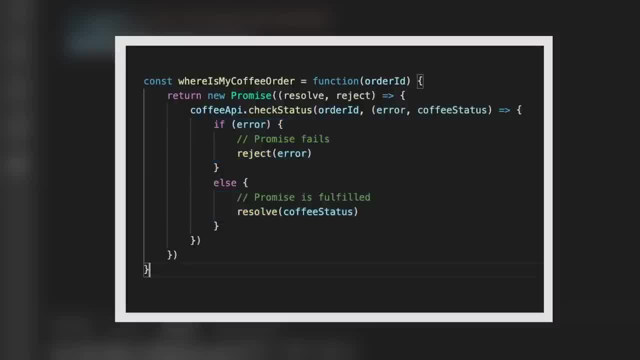 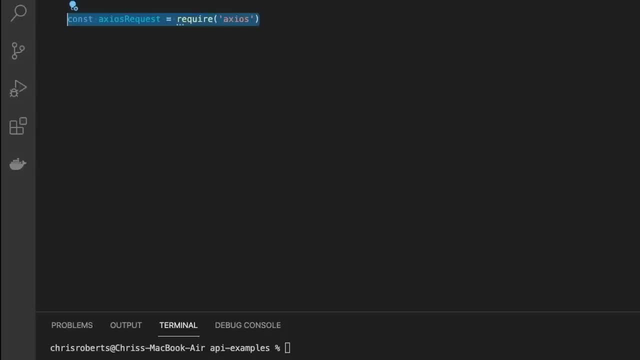 that the promise itself is actually resolved or rejected and you can use the result of that promise. So let's have a look at an example in JavaScript Now. imagine you were building an app that suggested things to do when you were working from home, and you were working from home. You. 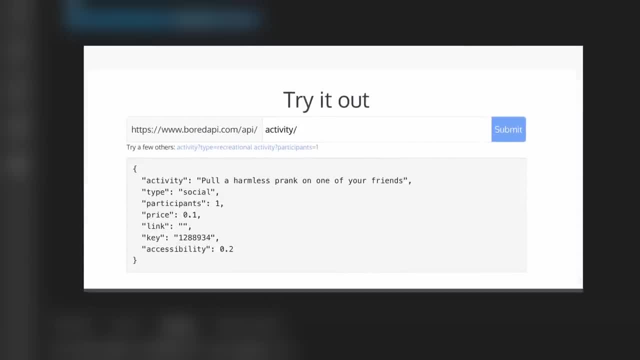 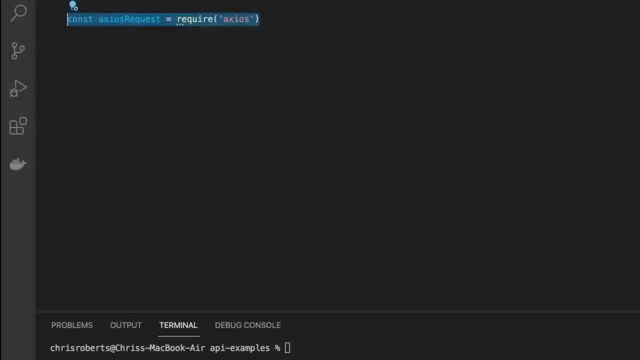 will be using the Board API, and the Board API just returns random suggestions of things that you can do, along with the number of participants required. Let's just keep it really simple by going to the API, getting a suggested activity and then logging out the activity to the console. 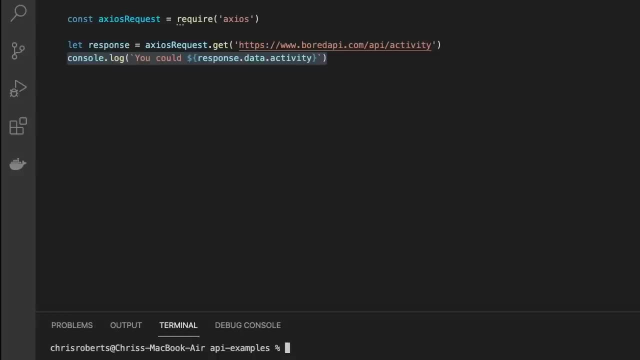 Now, in this example, we're using the Axios request library and the get method returns immediately, but that doesn't mean that the request has finished processing. What we have is a promise that the request will be fulfilled in the future. So this code will fail because the 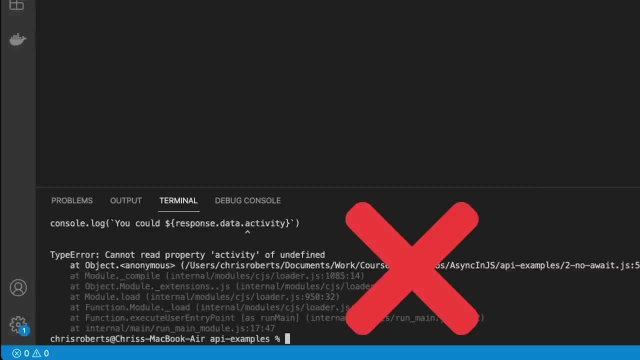 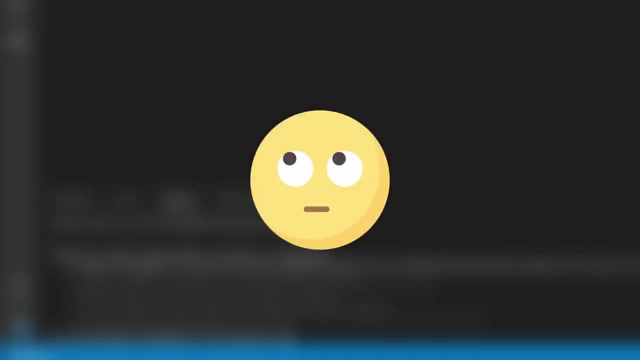 response object is not what we're expecting, so the data and activity properties do not exist. So is there any way for us to get access to the result of the request and run code when it returns? Well, thankfully yes, because JavaScript gives us a couple of ways to wait until a task. 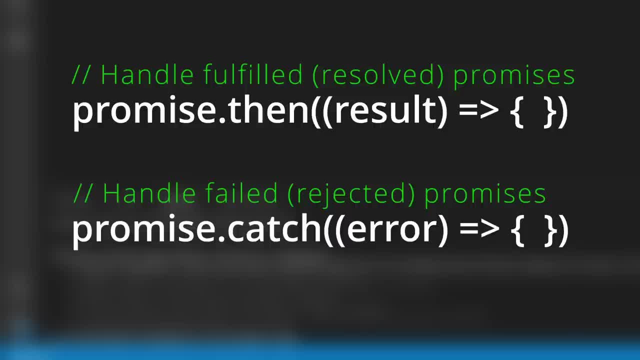 has finished and use the result or catch any errors that occur. The first way is by using a couple of special methods on the promise object. The first one is called, then Then is called when the task completes and as a parameter it receives the result of. 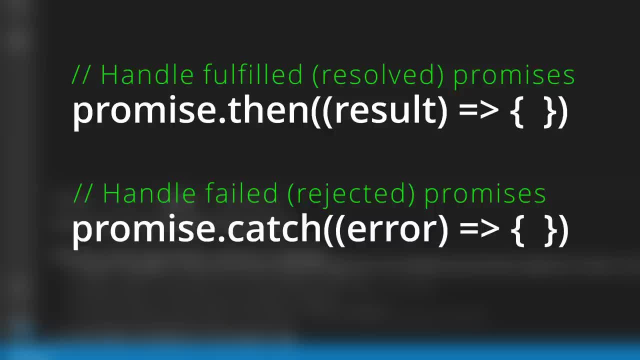 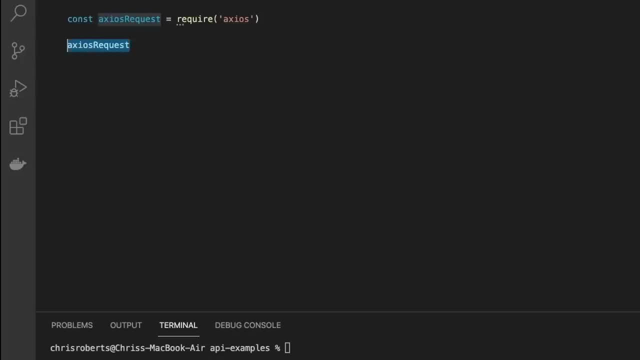 The catch method is called if anything goes wrong while processing our request, and this receives the error that occurred as a parameter. So let's replace this code, use the Axios request library and call the get method Now, because get returns a promise object, we can immediately chain on the then method. 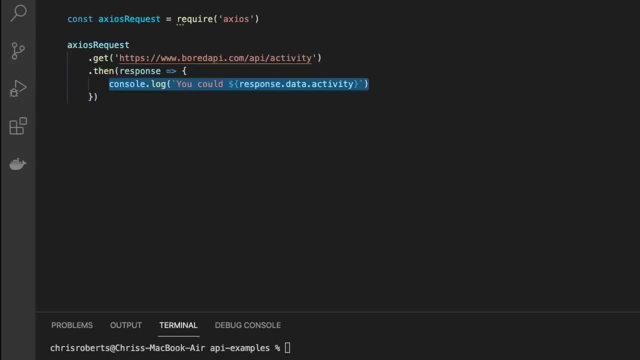 Inside our then method. we'll log out to the console the suggested activity from the API. Then after this, we can chain on the catch method. This will be called if anything goes wrong while processing our request, Let's just log in. We'll log out to the console the error message that is returned. 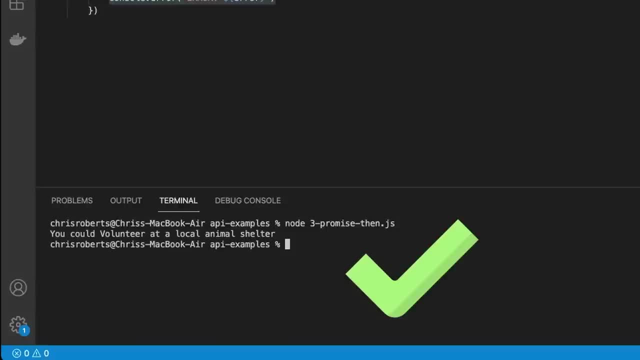 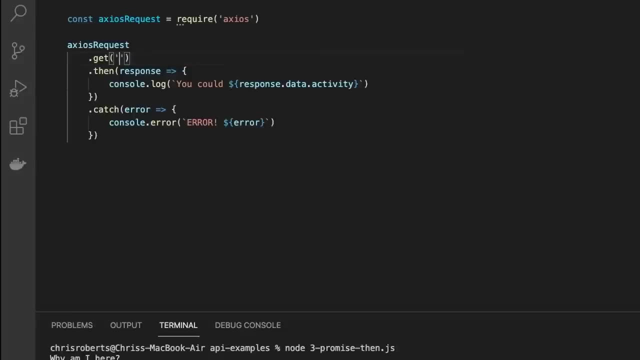 then we can run this and see that our console log executes in the right place. Now, to simulate an error occurring in our request, let's replace the URL with a call to the HTTP status API. This is really useful for testing different status codes, and we'll just request. 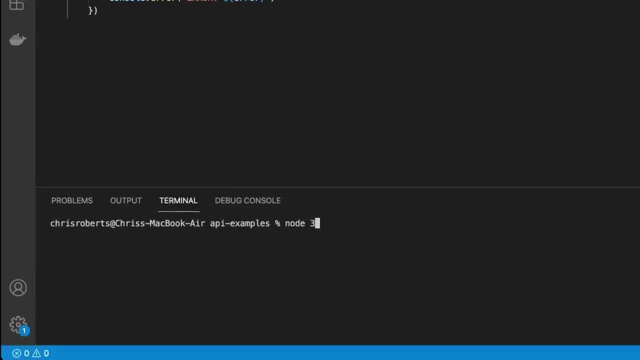 a 404- not found error, We can run this again and see that our error is neatly caught by our catch method and printed out to the console. It's worth noting that any code placed after this will be executed immediately. So if we put a console log here at the bottom. 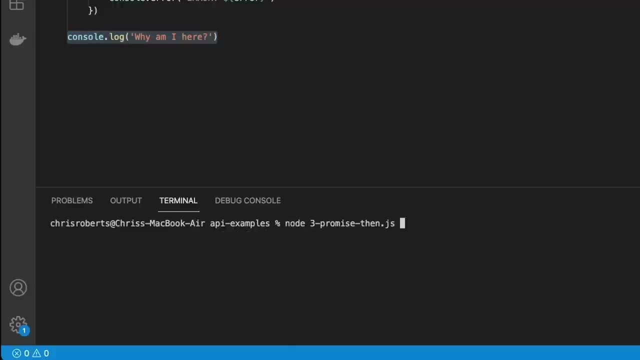 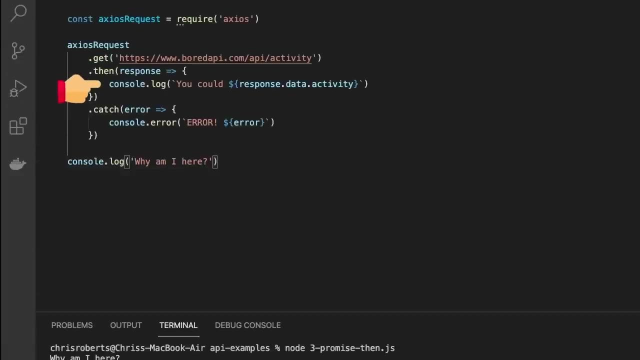 we'd expect it to be written out after our request returns, but actually it gets printed out first. This is because only the code inside the then and catch methods is executed after the request returns. Now this works fine. however, as you can see, the code isn't particularly nice to look at. 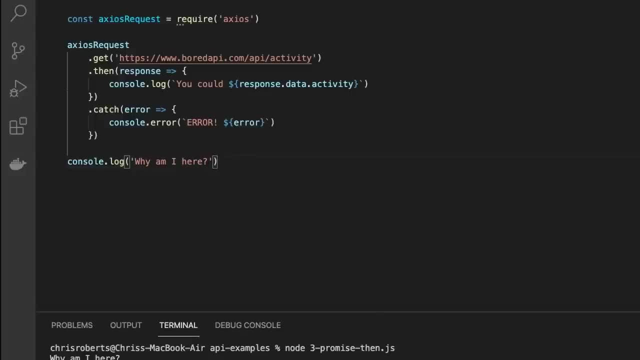 and if you had a lot of complicated code inside your methods, things would soon start to get quite unwieldy. So what we need really is a way of receiving the results of our promises sequentially, just as if we were doing this in a different way. So let's run this, Let's run this, Let's run this. 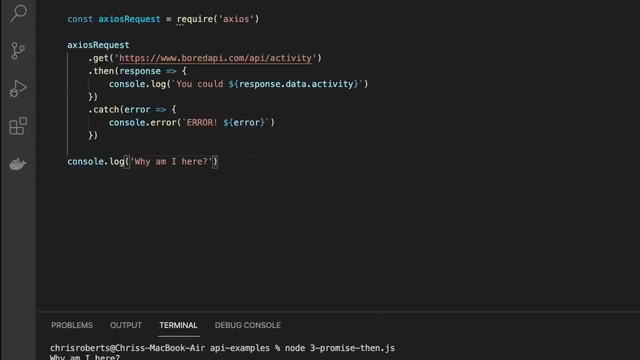 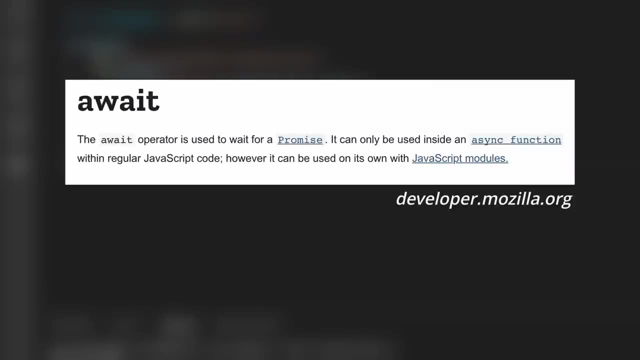 Just as if we were dealing with simple types like strings and numbers, And this is where the await keyword comes in, And await does exactly what it says: it allows us to wait until the promise has completed before moving onto the next line. This makes our code a lot neater and easier to read. 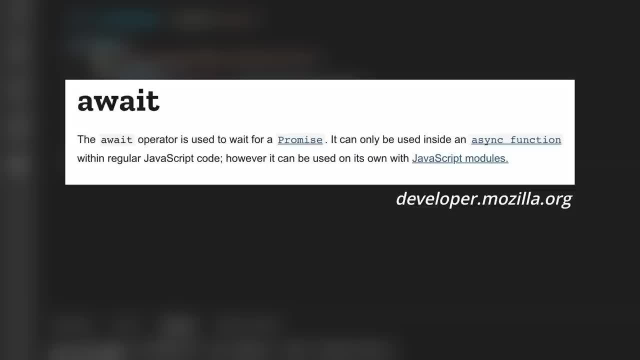 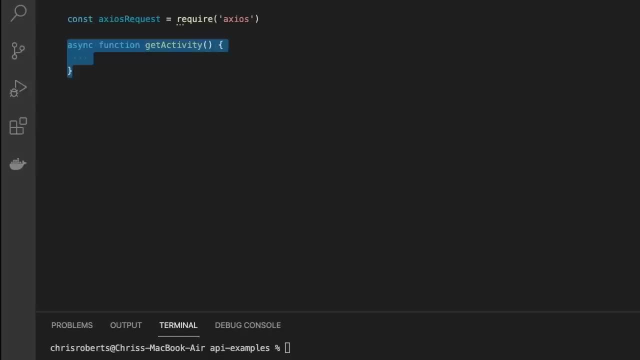 JavaScript requires that our await keywords be used inside functions marked with the async keyword. So let's replace our promise chain with a function marked with the async keyword. let's call it getActivity, and now we're going to make the same request to our board API. 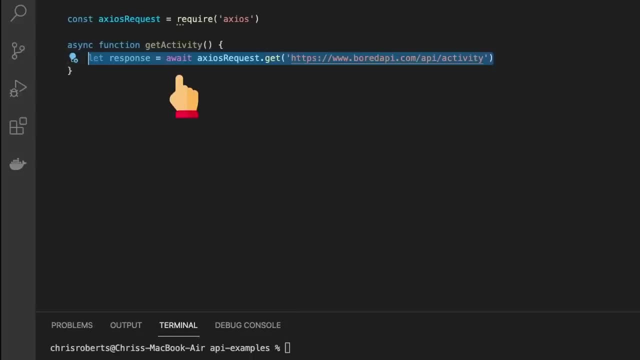 But notice we have the await keyword before the method call. Then immediately after, on our next line of code, we can use the response and log out to the console the suggested activity. This console logline will not run until the promise resolves or is returned. 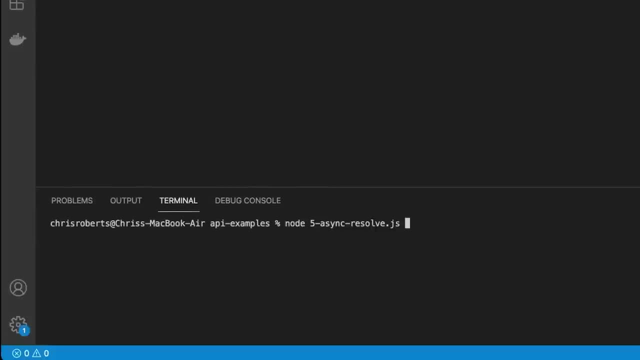 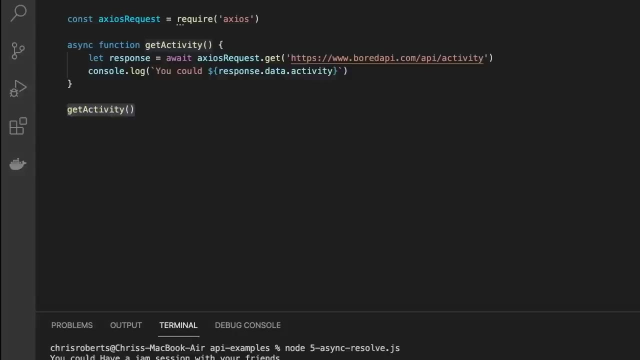 We can call our getActivity and we'll see that our code executes perfectly. Now, because the await keyword allows us to move this kind of asynchronous code back into the main flow of our app, we don't have access to this specialised catch method to handle any errors that. 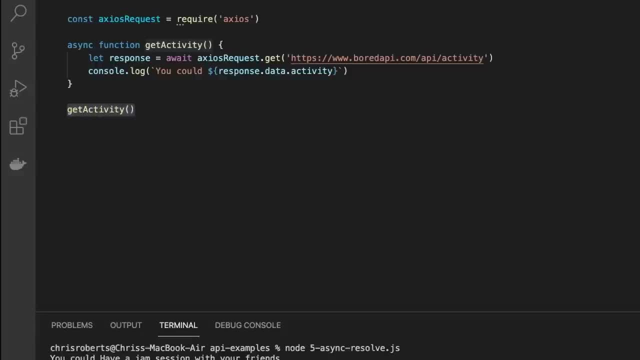 occur. So what happens if something goes wrong? Well, because our code executes sequentially, we can just wrap this with a normal try catch block Inside our catch method. we can just log out to the console the error. This time, to simulate a server error, we'll use the HTTP status API again. 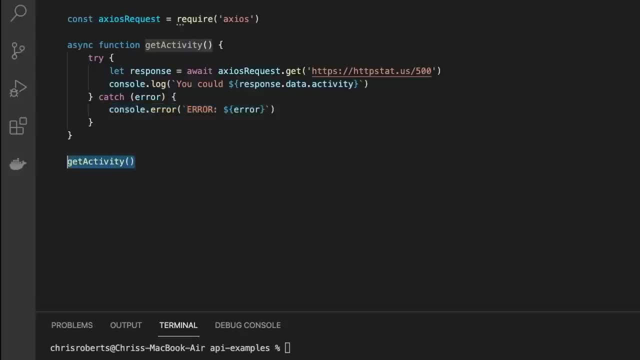 and this time we'll request a 500 server error. We'll call our getActivity Notice. our request error has been nicely caught and logged out to the console. I hope that has helped to demystify using promises and the async and await keywords in. 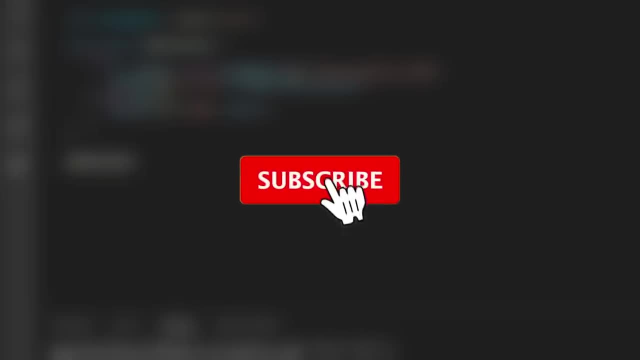 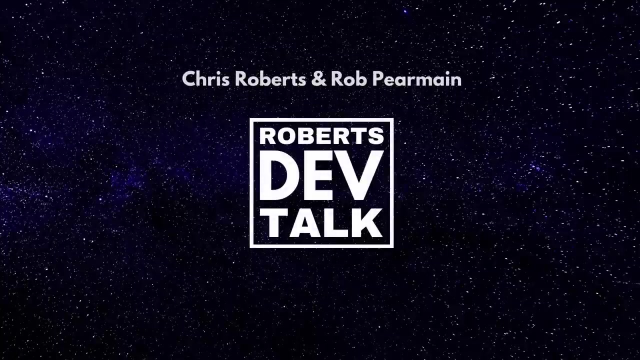 javascript. If you enjoy this kind of content, then we make videos every week, so make sure to subscribe and ring that bell icon so you never miss out on one of our videos. Thank you so much for watching and we'll see you next time.